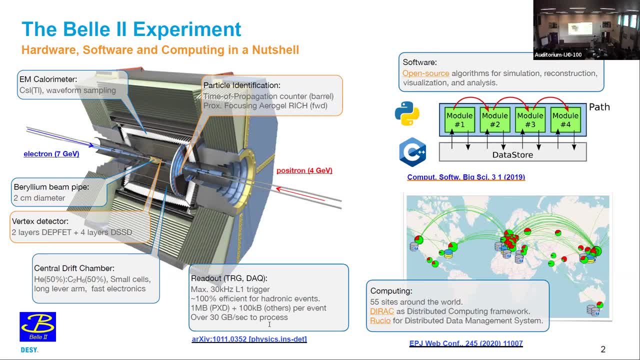 So that's why it's called a B factory, because we produce a lot of the mesons. All the readout has completely upgraded with respect to the previous B factory Bell and we are expecting around Well. the output of the readout is around 30 kilohertz in the full luminosity. 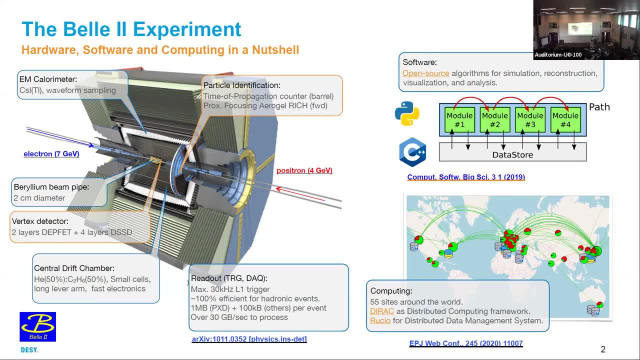 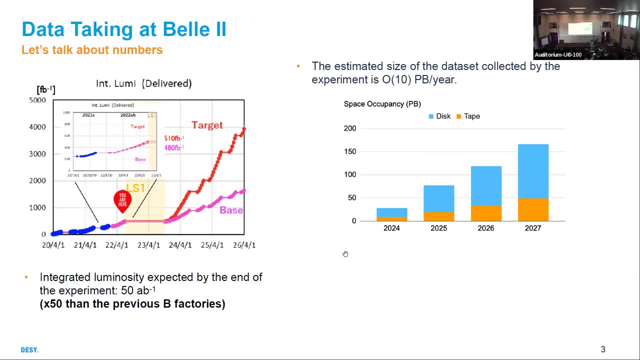 The software. I will talk a bit more about that in the next slides- And just to remark that we are using grid computing as all the LHC experiments. Now let's talk about the numbers. The interesting thing about Bell2 is the integrated luminosity. 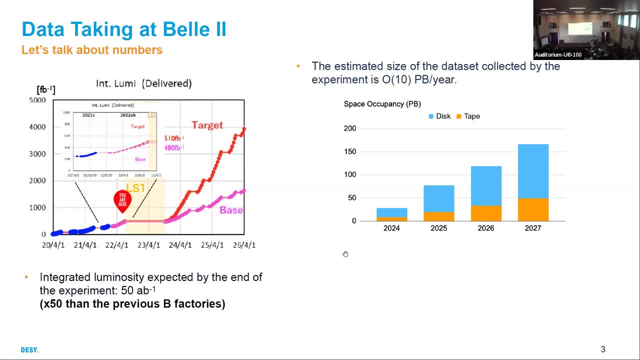 We expect to produce around 15 percent of iron at the end. This is 50 times more than the previous B factories. It's usually the number that we use to get out benchmarks And just to give you a little bit of an idea of what we are doing here. we are actually working on a lot of these experiments. And just to give you a little bit of an idea of what we are doing here, we are actually working on a lot of these experiments. And just to give you a little bit of an idea of what we are doing here, we are actually working on a lot of these experiments. 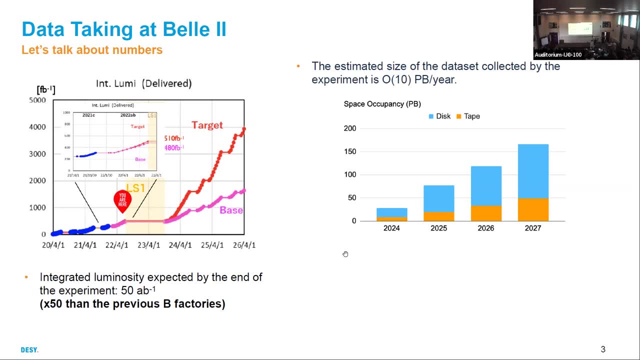 And just to say that the estimated size of the data set collected by the experiment is of the order of petabytes per year, So it's not as big as the high luminosity LHC. So that is not our challenge. But our challenge scales when you take into account the number of events, that corresponds to the luminosity that we're expecting. 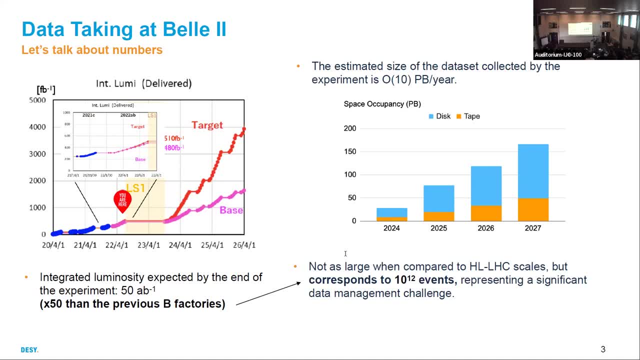 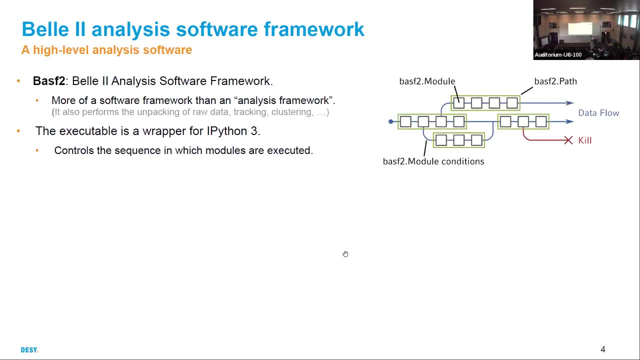 So that's what represents a significant data management challenge. Now, our strategy to reduce the data is not about removing objects, because the size of the events in the reconstruction is already small. It's mostly about the scheming. But in order to talk about the scheming, I have to say a few things about the software. 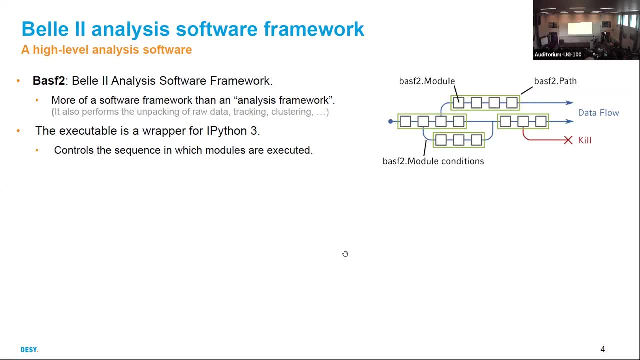 So this is our software framework. It's called BASF2.. It's well, it's from Bell to Analysis software framework, but this is more historical thing. But it does more things than just the analysis. It actually performs all the unpacking of raw data: tracking, clustering and so on. 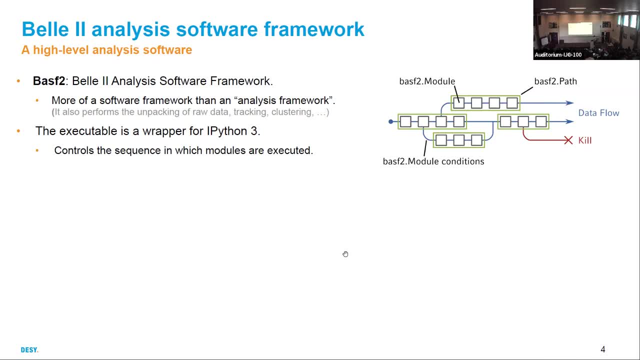 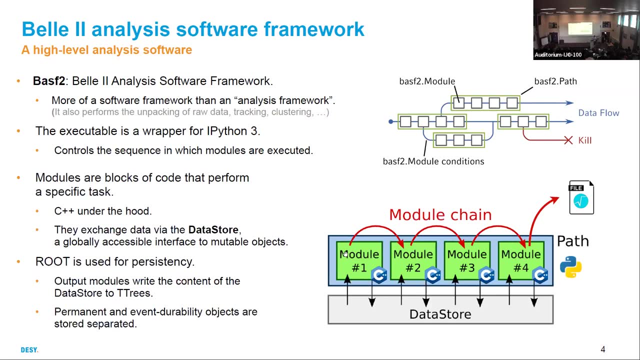 It's an executable, It's a wrapper from Python 3 and controls. It's a sequence in which these things called modules are executed, And these modules are just blocks of code that performs on a specific task. It could be, for example, well, some part of the reconstruction, some triggering, et cetera. 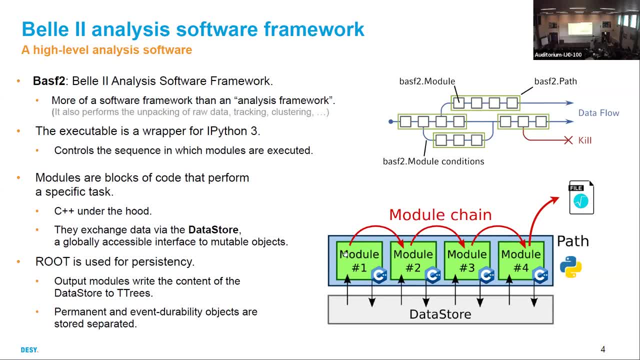 It contains C++ under the hood And it exchanges data via this data store. that is just a global, accessible interface to the objects in the modules. And well, root is used for persistence, So our data formats are actually based on root And the output is it's basically content of the data store into T trees. 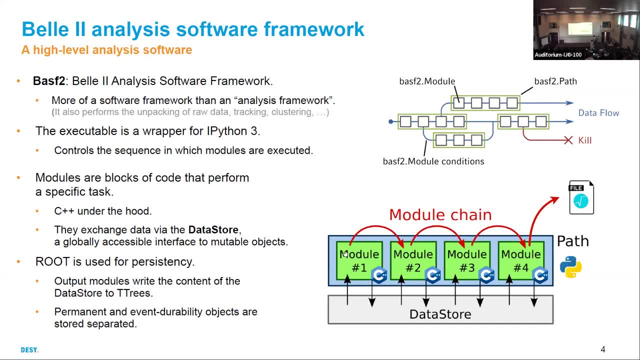 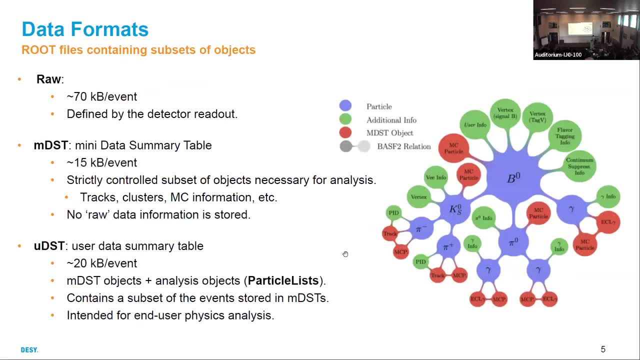 And well, it's separate, independently, permanent and event durability events. So that's what the software does, And let's move on to the data formats directly. So, as I mentioned previously, we have this thing that's called the mini data summary table. 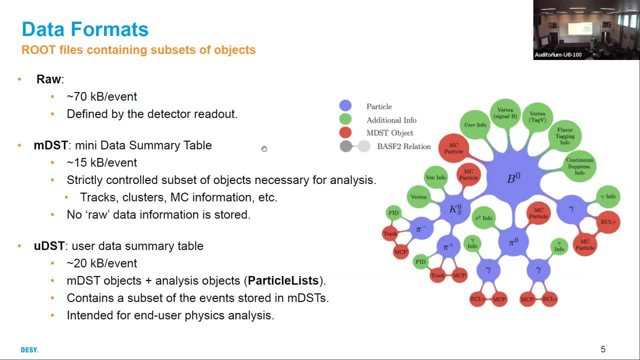 It's the output of the reconstruction And, as you can see, it's already quite small. So we are not dealing with the task of removing objects. However, we have still to deal with the number of events that people have to process, So this contains strictly objects that are necessary for analysis. 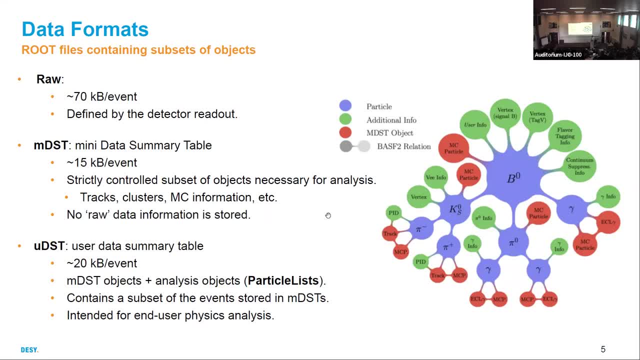 So no real data information is stored after the reconstruction And the format that is for end user analysis is the UDS team. So this is just user data summary table. It contains approximately 20 kilobytes per event. The reason why it's larger than this one is because we are performing the scheming of the events that are interesting for the analysis. 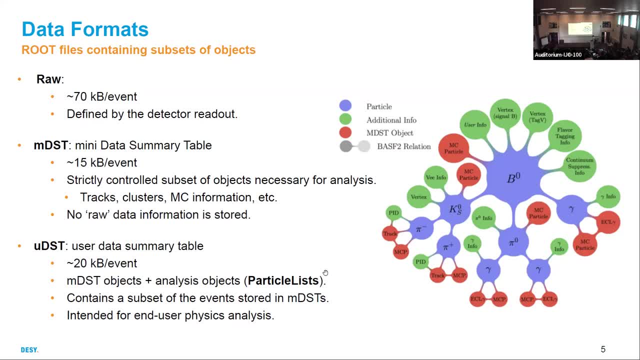 But additionally we include the objects that can be used for getting results. that is just particle. This is just a list of objects that represent particles and contains information of each one of the candidates that are reconstructing the events. OK, and this is just intended for the end user: physics. 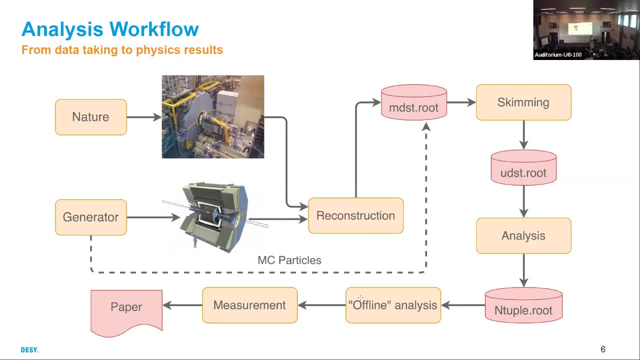 The workflow is pretty standard in Bell 2.. We perform very similar things going from the reconstruction to the MDST that I mentioned, And I will focus later into this part that is maybe the relevant for the session. So this MDST, as I mentioned, already contains just the objects that are used for characterised particles on each event. 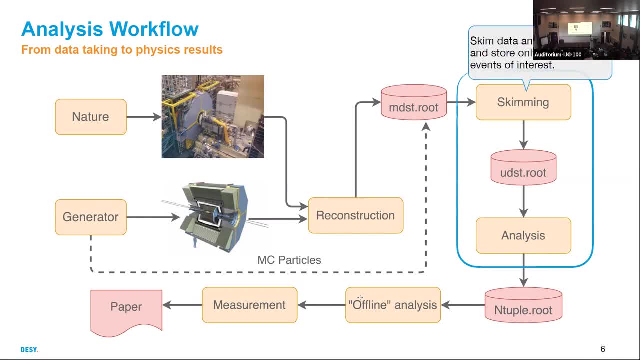 So when you perform the scheming, you reconstruct actually these particle candidates And then, based on that, you select what are the events that are interesting for your physics case, And this is the end user analysis. This is stored into this UDST. 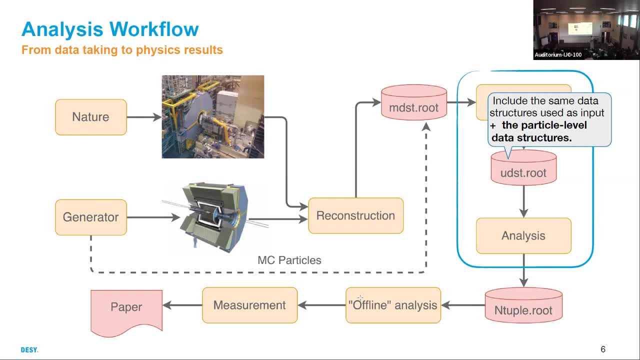 So after the scheming, including the information of the particle level data structure, So you get some gain into the CPU that will be used after all, because you don't have to pass through the process of reconstructing particle candidates again. But of course there is a small cost in increasing the size that you will use in the disk. 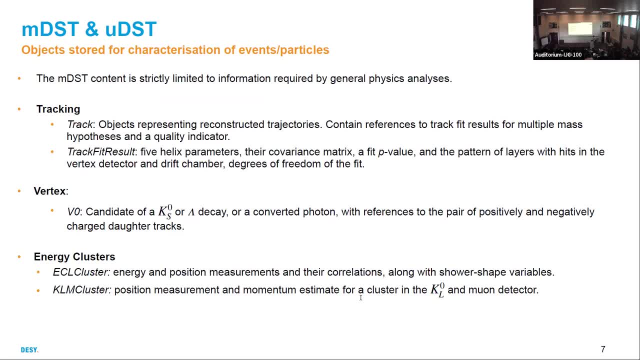 Now this is the list of objects that are included in this MDST and UDST formats. It's pretty standard, So I will not go through all of them, just to say that we contain the information of the tracking. So tracks and fit results, vertexing just to reconstruct B0 candidates like the shorts lambdas, energy clusters both from the electrocalorimeter and the KLM. 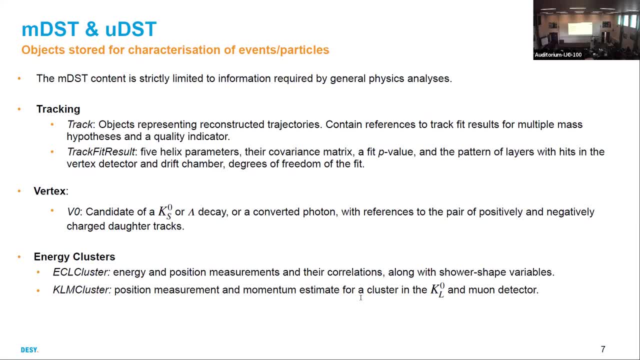 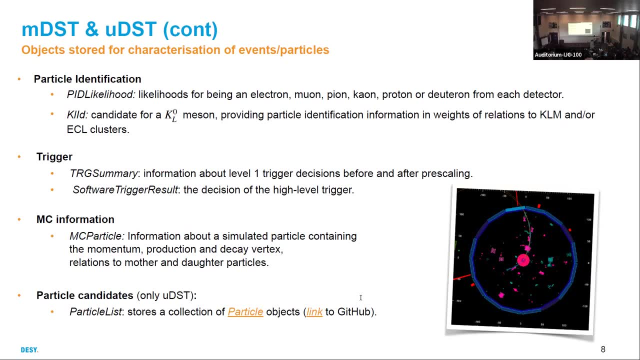 That is the last layer that reconstructs muon KL long candidates for particle identification objects. That is mostly the likelihood of the different sub detectors for reconstructing particles triggering information and Monte Carlo It's. it's also a story. So for MC matching and the well, the, the interesting one probably for this talk is the particle candidates that are stolen. UDS team. 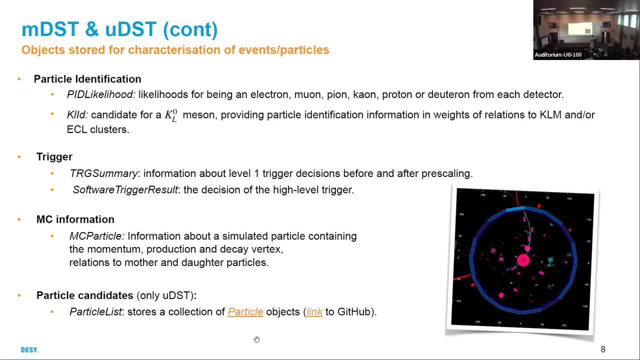 So this is the, as I mentioned, the collection of particle objects that if you want to go to the definition, you can click here and they send you to. to get up, And this is the definition of this particular subject that we use for performing the analysis on candidate base. 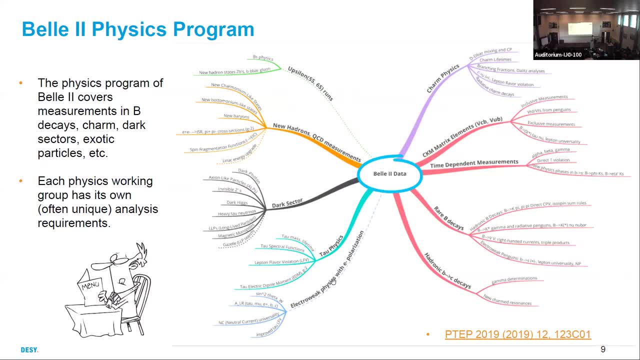 Now the physics program at Bell tool. let me just say a few words about it because it's relevant for the discussion. We just don't, We don't do B physics, but there is quite a long list of analysis that they're being performed right now. 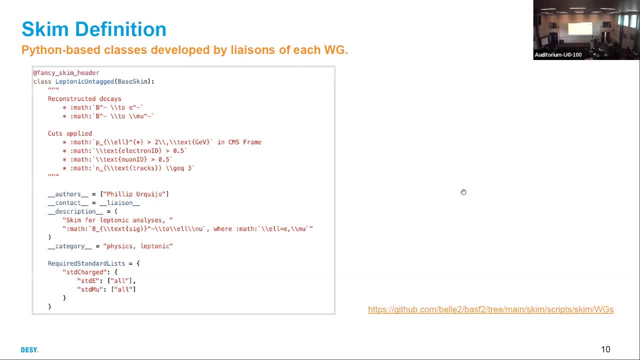 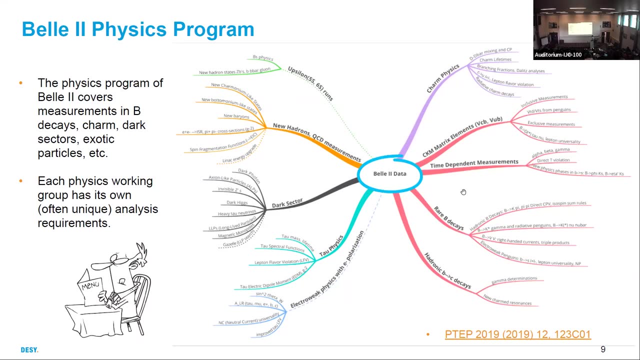 So this part is just what covers the B physics, the B physics in in in our program. But we also have charm, searches of new hadrons, exotics, dark sector physics, And we can extend this if we have the capability of running in UPS, you know five or six or electric. 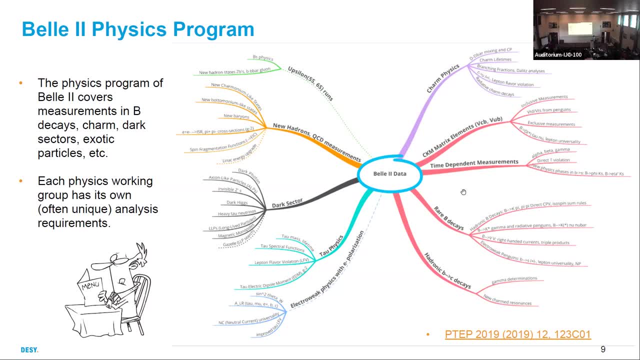 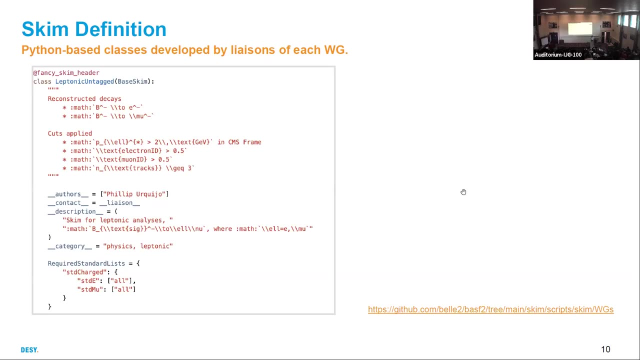 And the important thing here is that each physics working group Has its own, often unique, analysis requirements. So that's when we start to deal with different, different requirements that will be defined for the, for the scheme. Now let me talk about how the scheme is defined, about two. 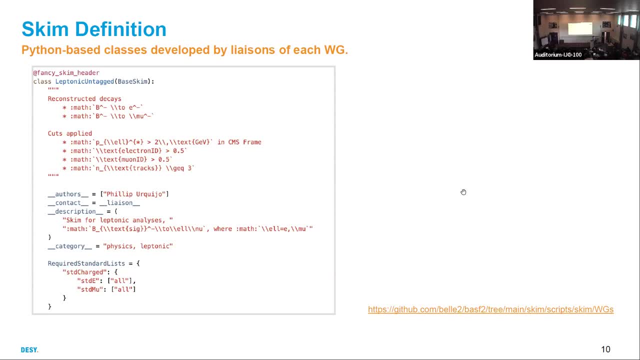 I think this is a pretty cool feature of the framework and it's quite easy to do it. maybe too easy And that's a problem- I will talk about that later- But the thing is that the analysts were the working groups in this case- just defined some metadata. 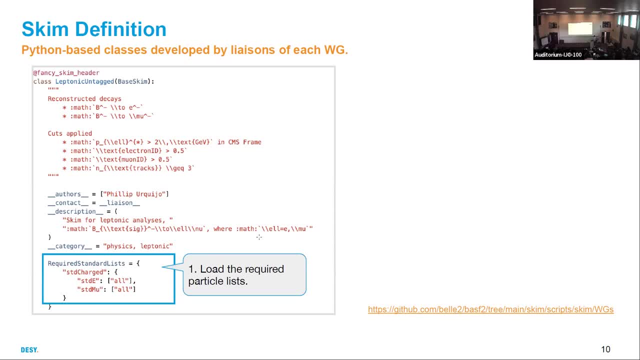 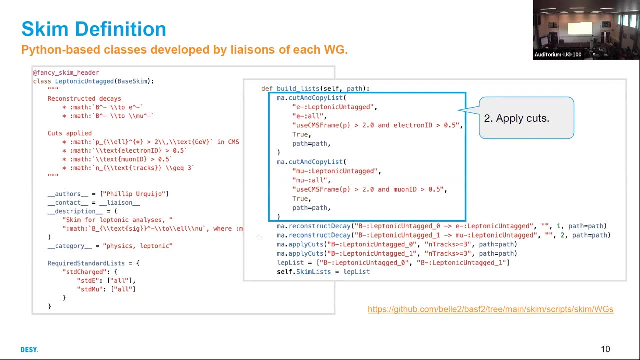 then load the standard particle list that are required to analyze the kind of events that you are interested with, then applying some cuts into the particle list that you have just defined, Like, for example- in this case it's just electrons, muons- and then apply the selection using this declarative format: 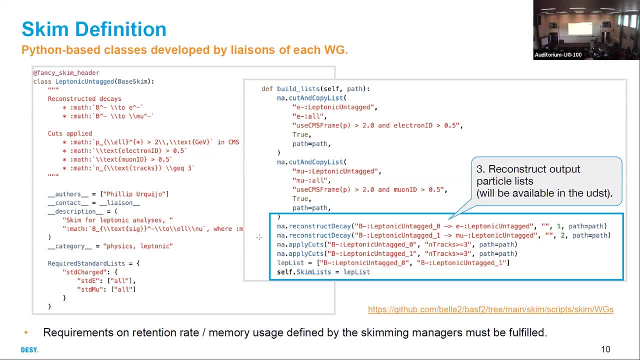 and finally reconstruct the output particle list that will be available in the UDS team. And all this is just. also, you can apply additional cuts into the particle list depending on what is the kind of things that you are interested, And that's it. 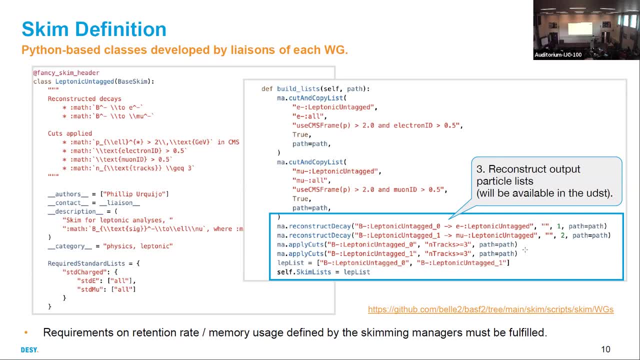 So this is the definition And then, once it's done, you can put it in the repository and then it will be processed on grid. It's super easy, I would say, And just you have to fulfill some requirements on retention grade, memory usage. 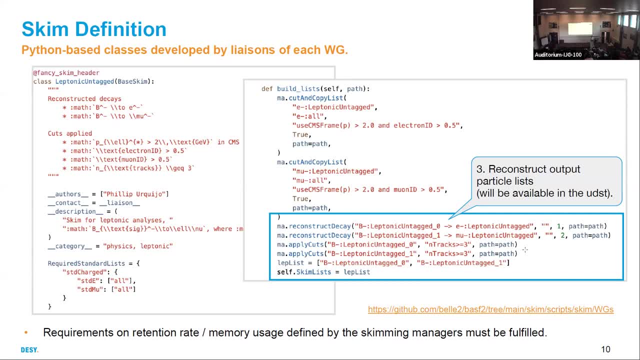 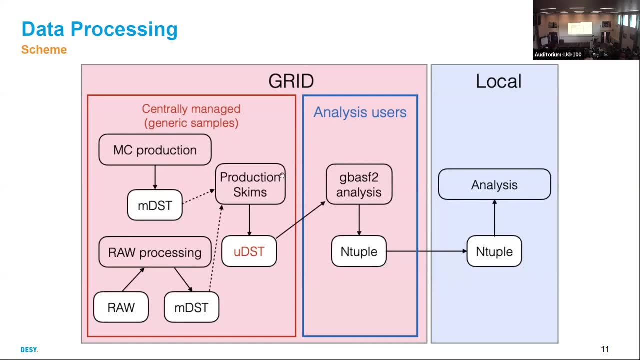 that are defined by the managers. It's mostly dependent on the limitations of the sites. So the scheme is that, once you have the definitions, this is centrally produced by this production and schemes that produce the UDSD, And the idea is that the analysts use the grid. 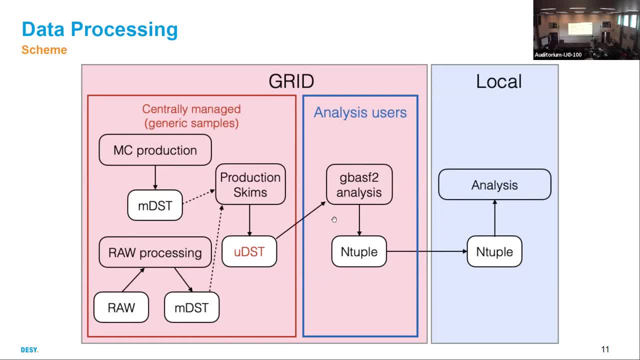 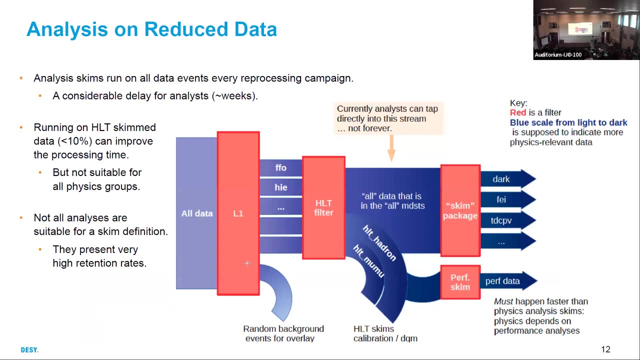 to access this UDSD format to get the intervals and then get the final result. So the framework itself, I think, works great. The problem is when we move towards the scalability of this thing, and that's when the problems start. That is probably where we would like to get some ideas. 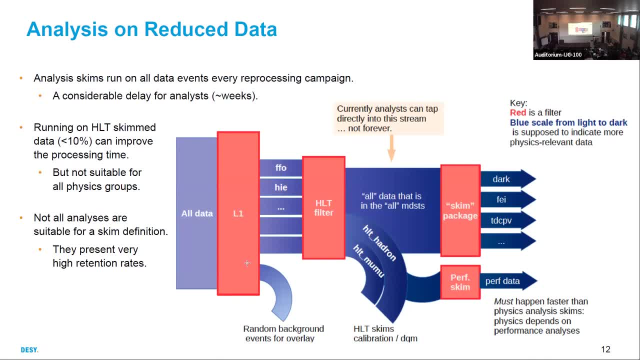 All right. so this is the process of data reduction, Again pretty similar to what has been shown already. One of the first problems that we have seen is that the analysis schemes runs on all data events, every process campaign, So this represents considerable delay for analysts. 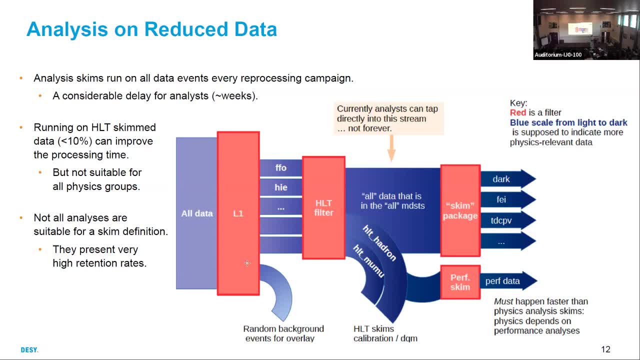 In particular, since we are ramping up the luminosity. people want to analyze data now, but this is sometimes not possible, So many of them are actually analyzing into the non-scheme stream, which is, let's say, okay-ish right now. 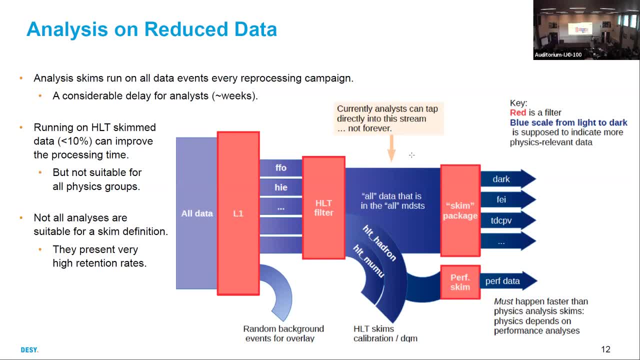 but as we increase the luminosity this will not be possible anymore. So one idea is that we also have defined at the HLT level some schemes that in principle are intended for calibration. Some people can actually use these ones for performing analysis, So the scheming in principle could be done. 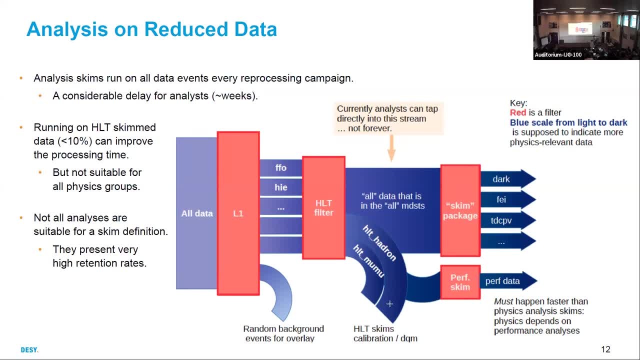 for example, in this one HLT Hadron. that is basically trying to identify hadrons in the event, but this is not suitable for all physics groups. It's just a partial solution And one of the big problems is that not all analysis. 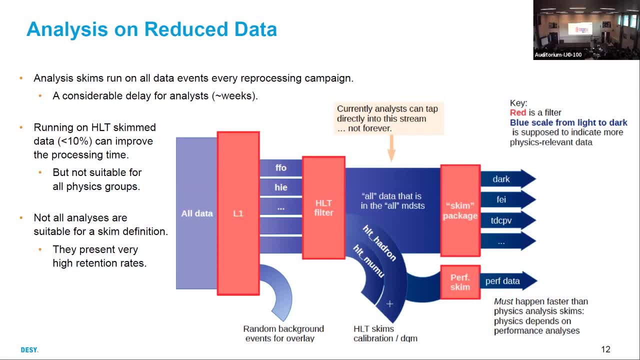 are suitable for a scheme definition, And one of the big problems is that not all analysis are suitable for a scheme definition, And one of the big problems is that not all analysis are suitable for a scheme definition. They present very high retention rates, Thanks. 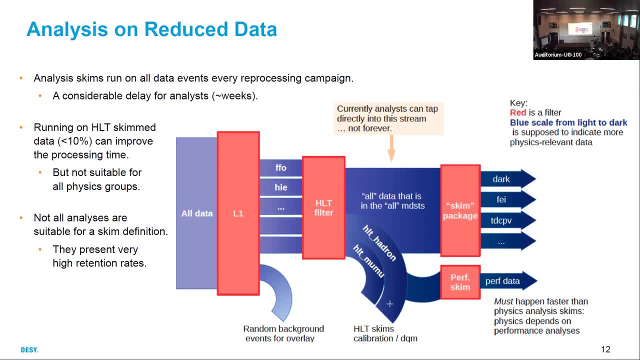 So if, for example, you are trying to find- I don't know- a bump coming from two tracks into your band, then we are pretty much making a copy of the full data set. Well, once the scheme package gets the output of the different requirements of the physics groups, 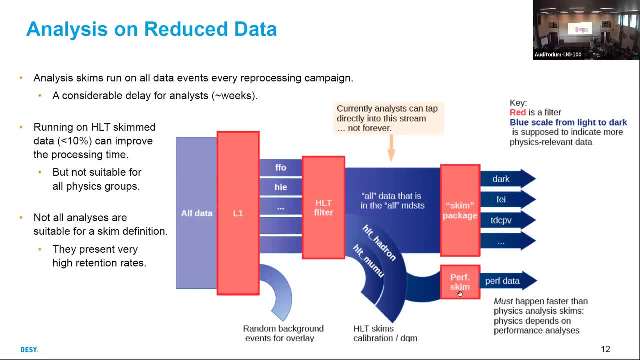 in principle, they must be analyzing this part. Plus, we have what is called the performance scheme And this, in principle, must run faster. They actually come from this stream of already HLT well high level trigger scheming. 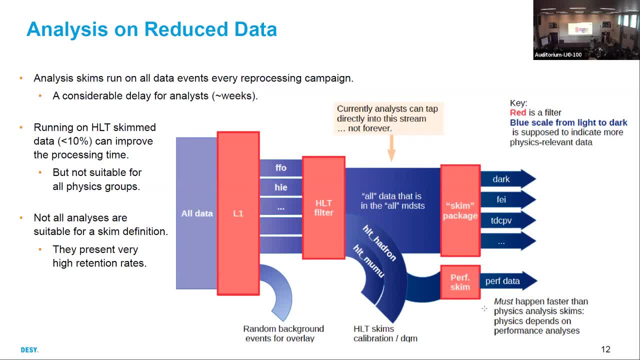 And the idea is that these files must be faster available, because they're the ones that are intended for getting the performance, the systematics, and they must be in place by the time that the data actually comes here. So the final goal is plugging this into machinery. 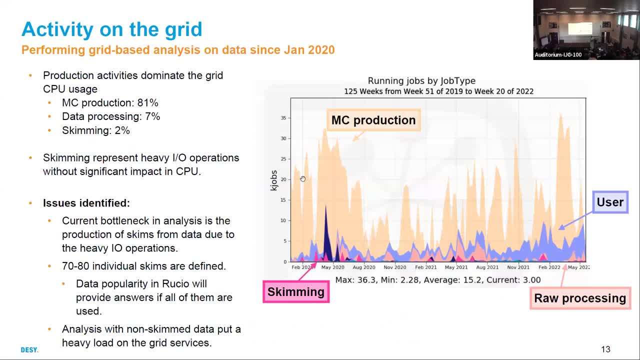 that automatically gets most of the systematics. Well, the the activity on the grid. just to mention that the scheming does not represent an impact into the CPU usage. it's mostly heavy IO operations And, as I mentioned it already, one of the big problems is the delay. 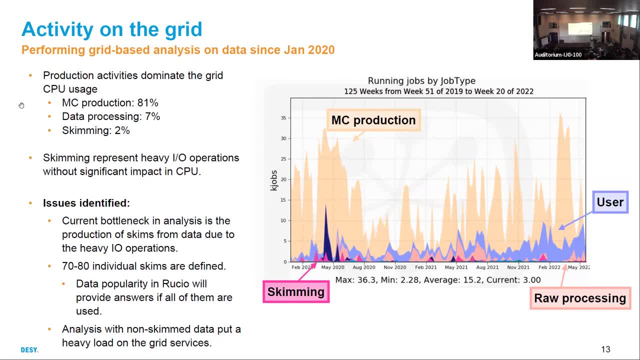 of the production of the scheme, given the data, this heavy IO operations. And another problem that was already mentioned in Atlas and it actually triggered an alarm in my head is that we have 70, 80 individual schemes and it actually triggered an alarm in my head. 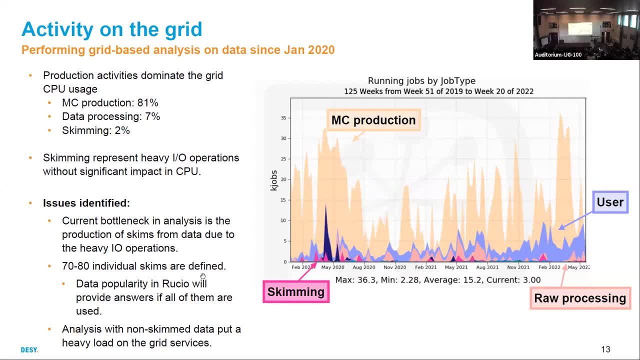 is that we have 70, 80 individual schemes, and it actually triggered an alarm in my head is that we have 70, 80 individual schemes defined. It's just by the requirements of the groups. as I'd say, defining a scheme is just, it's quite easy. 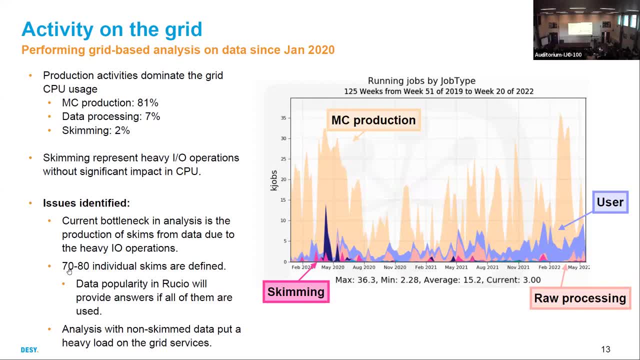 Then we don't know really if we. I mean, the idea would be to reduce this and data popularity in Rusio. now, Rusio, it's used as a distributed data management system, So the popularity in Rusio will provide answers if all of them are actually being used or not. 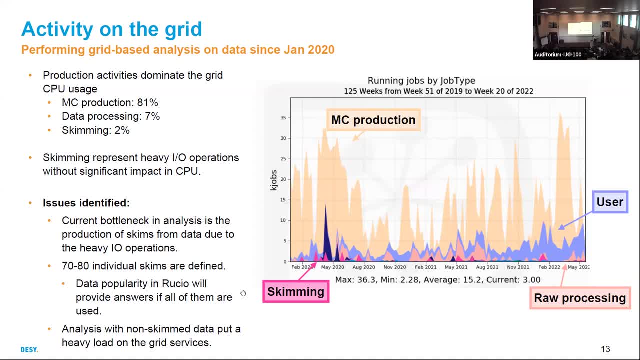 And, if not, just have a word with these groups like: hey, when you define a scheme, you are not using it. what's going on? And well, the analysis with non-scheme data would heavy load on the grid services. 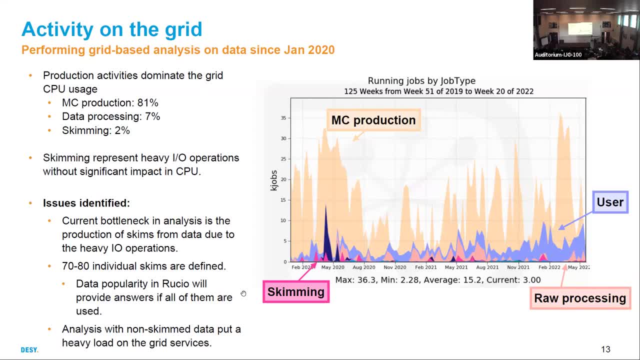 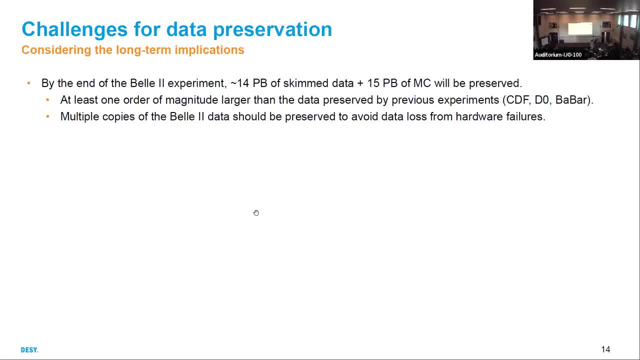 So right now, the scale is okay, as I said, but as we increase the luminosity, this will become more and more a problem, So we have to solve this eventually. And finally, I would like to say a few words about the long-term implications for data preservation. 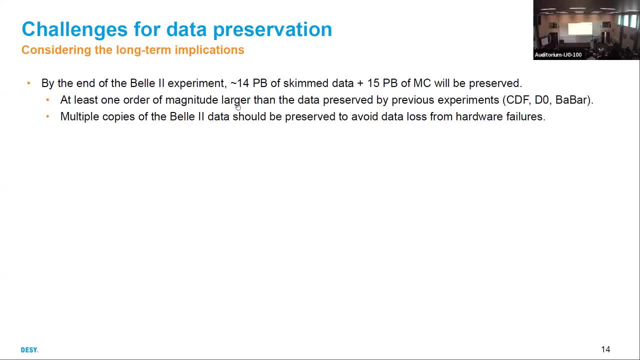 So, when you take the numbers at the end of the built experiment, we expect around 40 petabytes of scheme data- not similar size of Monte Carlo, but similar size of Monte Carlo but similar size of Monte Carlo that has been. that must be preserved. 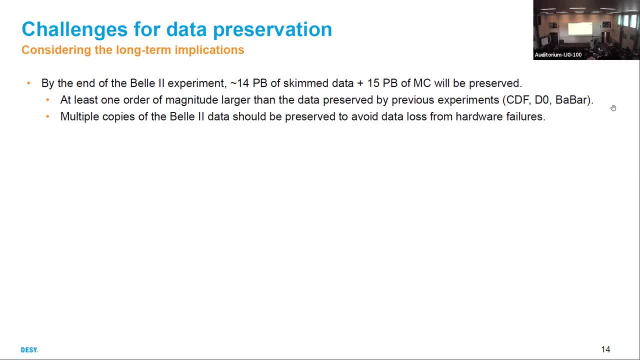 This is more or less an order of magnitude larger than the previous experiments that we have been comparing with the CDF, the 0-bar And, of course, multiple copies should be preserved to avoid the data loss from hardware failure. So this is relevant because well. 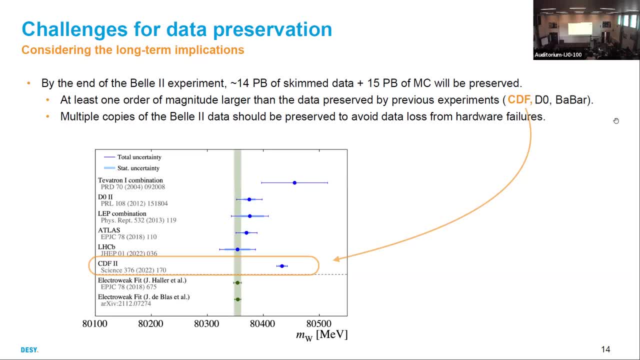 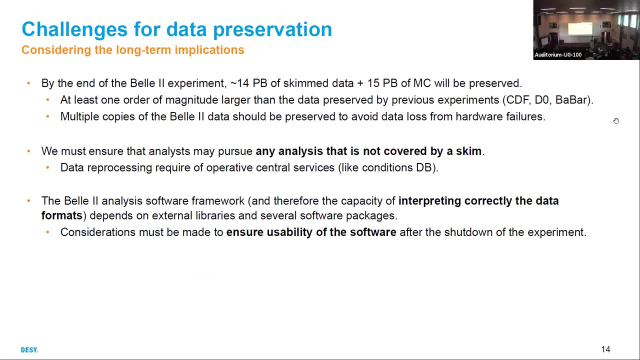 we had a reminder a few days ago about why this is important to have access to what you would call legacy data- And I think it's a relevant topic to discuss, And since this is an excellent forum to do it, so we must ensure that analysts may pursue any scheme. sorry, 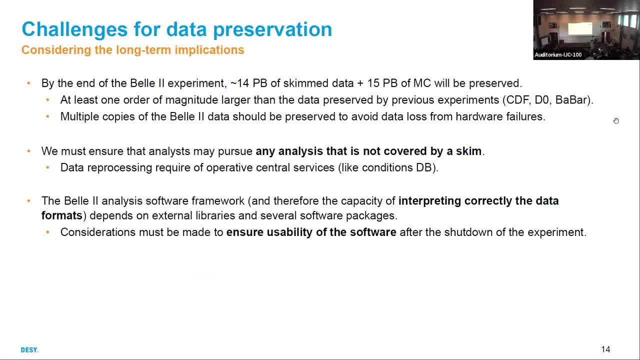 any analysis that is not covered by a scheme. That's more or less in our current situation that data processing require of operative central services, like conditions database, that are needed to correctly interpret what are the objects located inside these formats of Bell2.. So the analysis software framework depends. 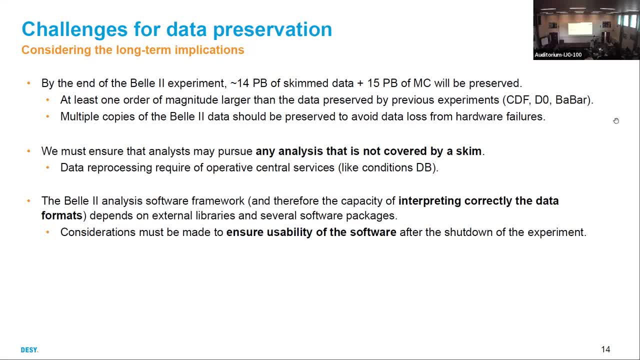 on external libraries and several software packages, And the considerations must be made to ensure the usability of the software after the shutdown of the experiment. So we consider that broader discussions about the feasibility of the long-term data analysis would be valuable for the high-end physics community. 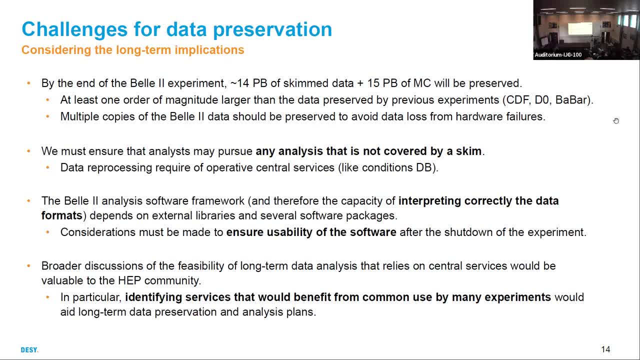 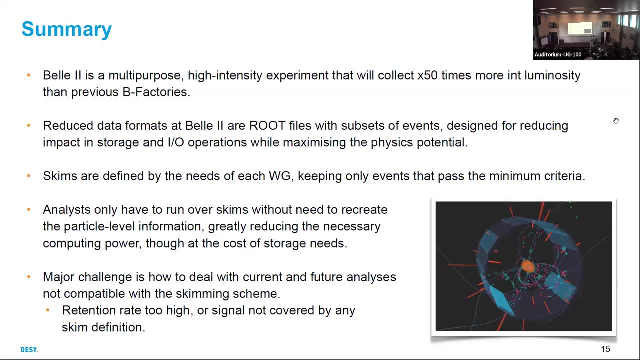 In particular identifying services that would benefit from common use by many experiments. So this will help a lot. So that sends to my summary. So the Bell2,, as I mentioned, is multipurpose- is a multi-purpose experiment. that means that we have many requirements for the analysis. 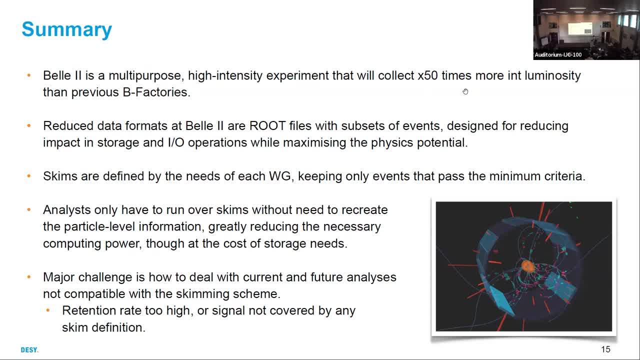 And we will collect 50 times more than the previous B factories. that scales the challenges that they had in the past. The reduced data formats are basically based on routes designed for reducing impact in the storage and in IO operations. Well, the schemes are defined. 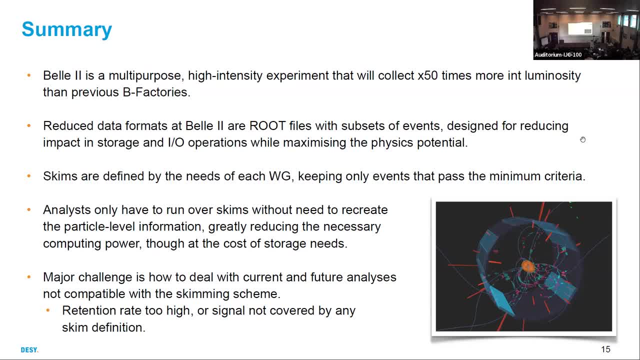 by each working group already mentioned, And the analyst. the idea is that the analyst runs runs over the schemes without the need to recreate the particle level information. I think this is a really nice feature And the major challenge is how to deal with the current. 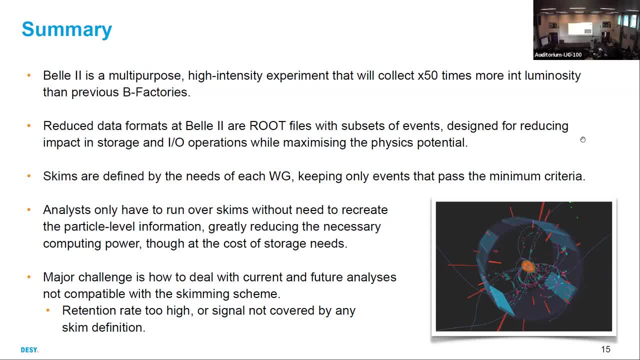 and future analysis that we don't have yet in mind, that are not compatible with the scheming. So just because the retention rate is too high or the signal is not covered by any scheme definition. So that's it from my side, Thank you. 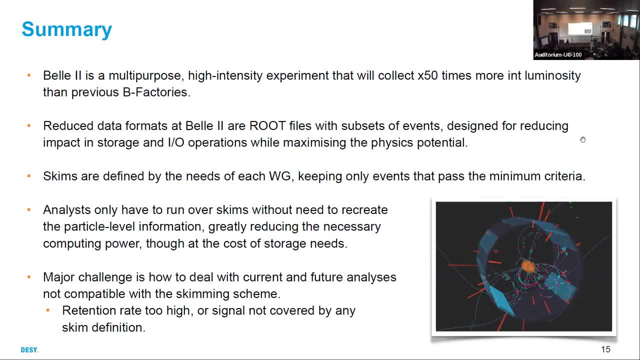 Thanks a lot. No questions on the screen. We'll see you again soon. I I see I don't see any hands or other questions in the room. There's one, Mike Sokoloff. Page three has projection. Page three has projection. 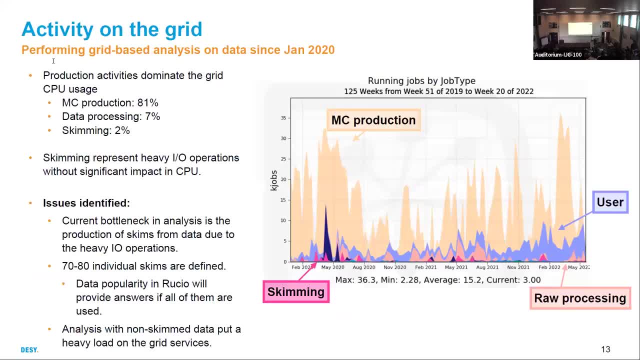 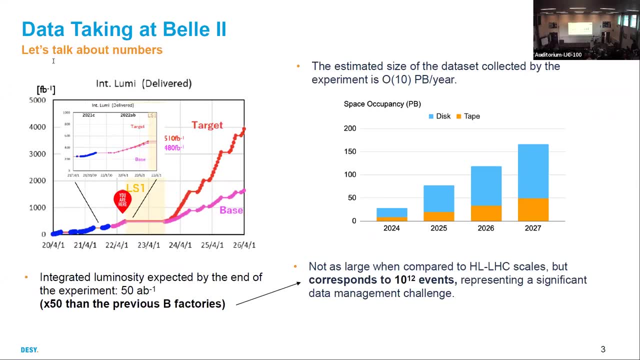 I'm trying to understand whether that projected luminosity is. you've got your data on tape on the right, You've got projected luminosity on the left. At what point do you expect to to accumulate 50 inverse out of Barnes? And is that really five inverse out of Barnes? 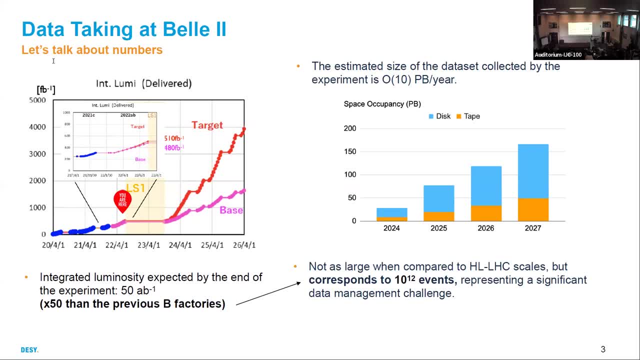 that you're talking about accumulating by 2027, or? Yeah, that's? Because there's there's a big difference between five inverse out of Barnes of data in the next five years and 50. Yeah, yeah, that's that's, that's true. 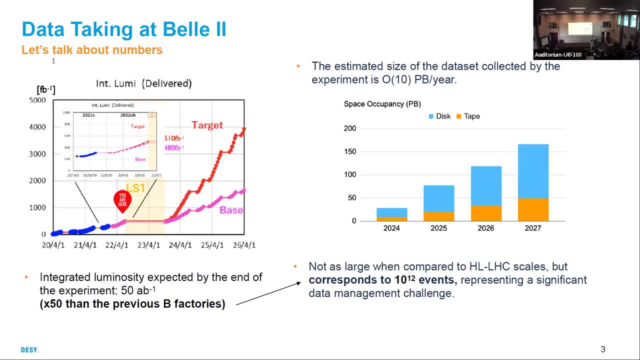 And actually it depends on how the instantaneous luminosity can be increased. So the projections so far have been right now puts officially until the 26.. And well, the goal of the 50 inverse out of Barnes is still on the table, But it's it's probably beyond 2027. 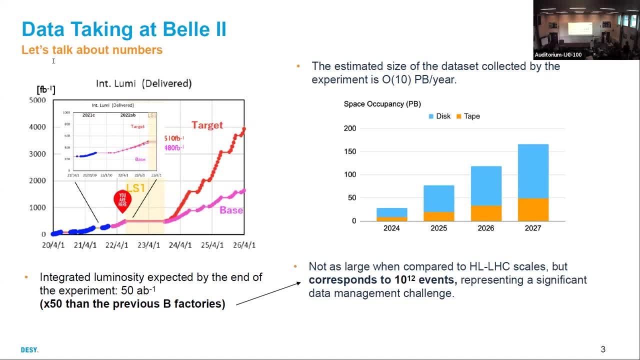 But it's, it's probably beyond 2030.. It's, it's just a matter of how, how, how much you can increase instantaneous luminosity. I don't know if Paul wants to comment on both of them, You can comment a bit, but yeah, 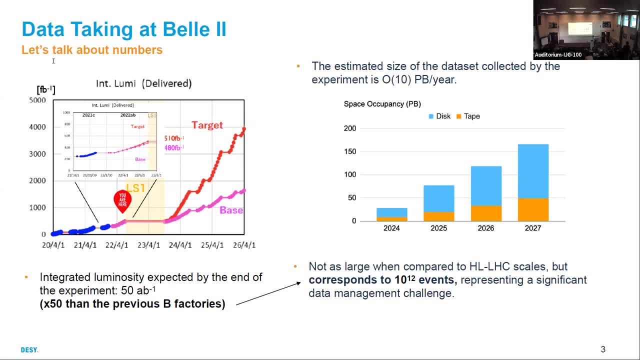 there's supposed to be an accelerator upgrade on that timescale, So just after the end of this spot. But the yeah 50 inverse out of Barnes is on a timescale of a decade or a bit more than that. It's challenging. 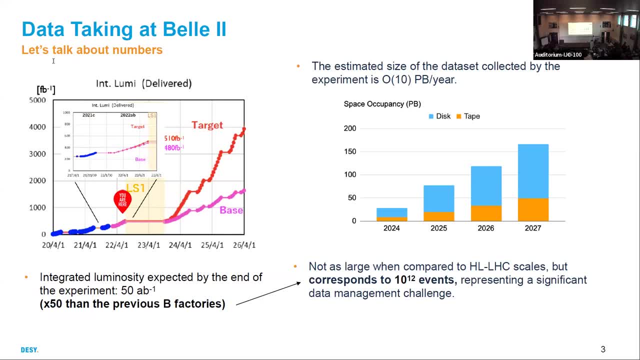 Any more questions. Not a question, but a comment. Thanks a lot for mentioning the data preservation impact of the simplified data formats. You're probably aware of PPHAP and the activity between other experiments happening in that area, And I think we are looking for someone from Bell. 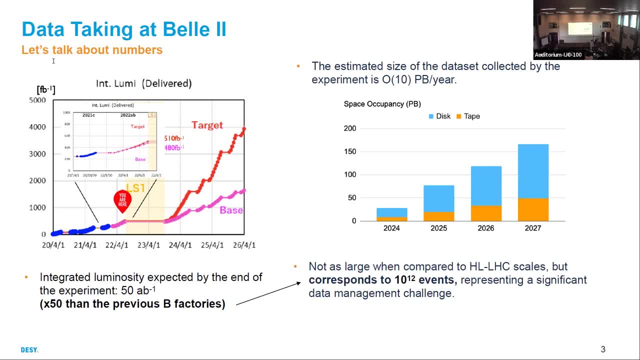 to contribute to this year's status update. So you know, I can only invite you to contribute what you saw also to them. Thanks a lot. Yeah, it will be very interesting. I'm just getting jump into this kind of discussion. 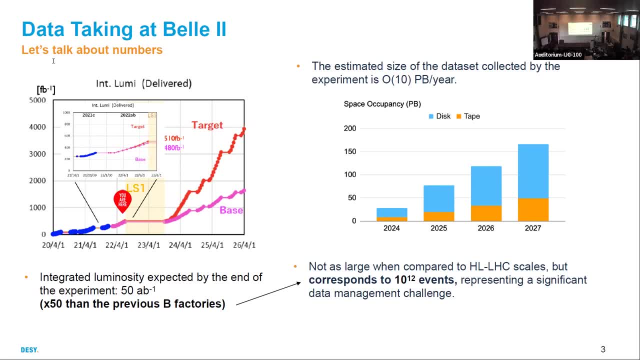 There is already a task force inside Bell 2 that is discussing this And I just jump into this boat to discuss from the computing point of view, in particular in my case. But yeah, it would be great if we can have some activity together. 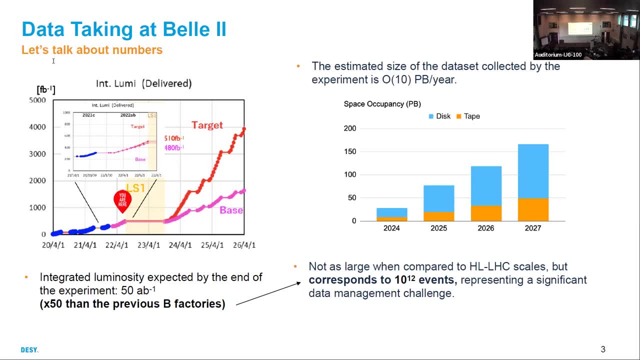 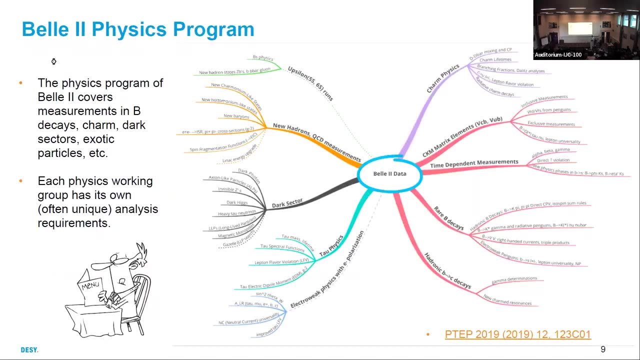 Maybe it's not just me, but other people. So yeah, Let's exchange the contact. Thanks, More questions. I had one. You talk about these different schemes. Roughly how many are there? Yeah, I mentioned that there are like 80 right now.